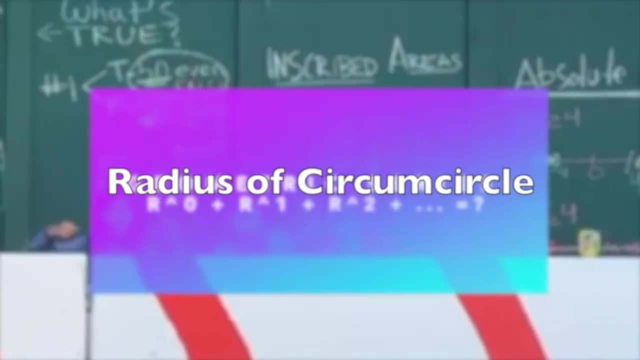 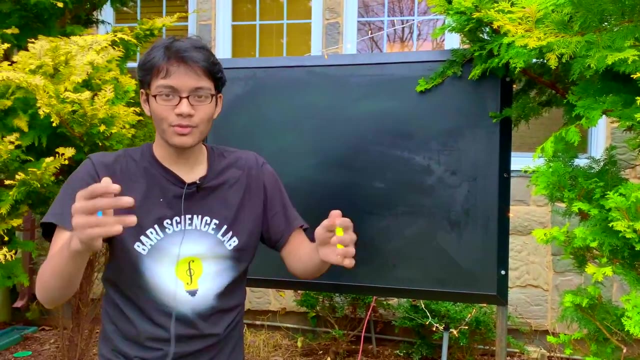 Alright, folks, welcome back to the next episode of Maths for Bronze. Wake up, bronze, wake up. Welcome back to the next lecture of Maths for Bronze. Today we're taking a look at the circumcircle of a triangle. Let's start with the triangle right. 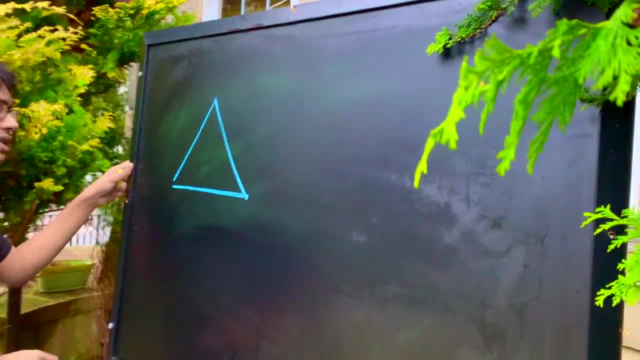 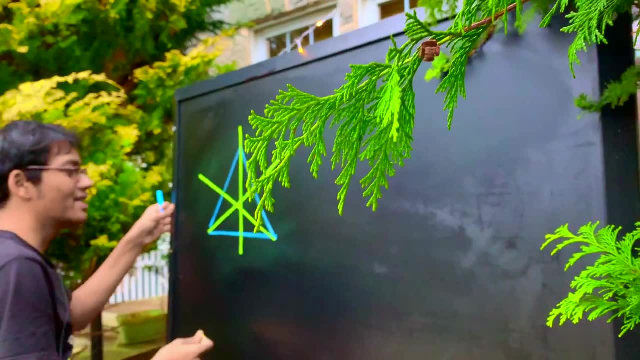 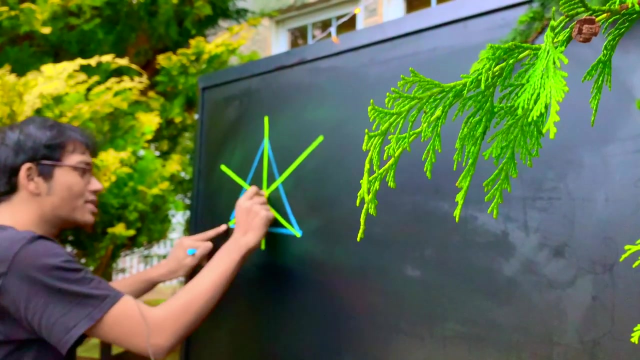 here And here's our equilateral triangle. To find the circle that encompasses this triangle, we're going to draw the perpendicular bisectors of all three sides where these three bisectors meet up. That's the center of our circle, And now we can use this segment as the 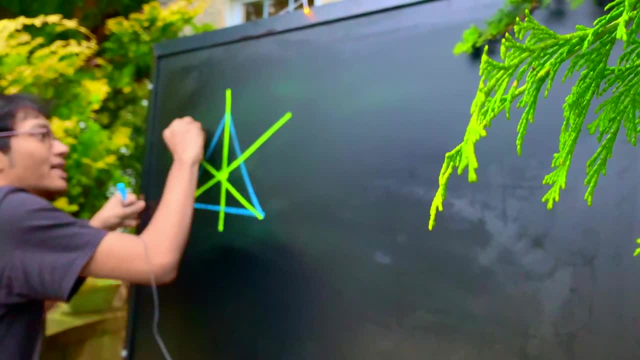 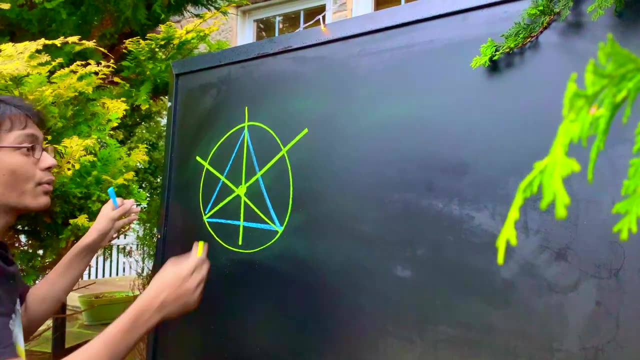 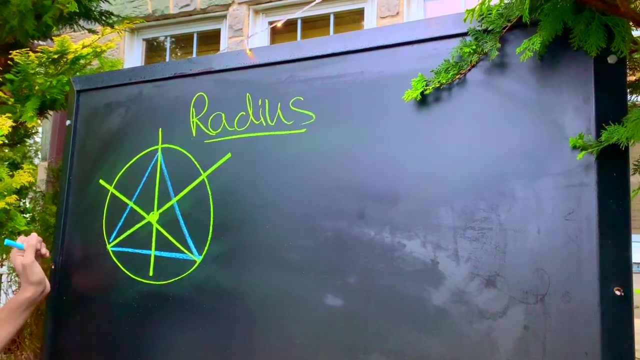 radius of our circle, of our circumcircle, rather and draw the circle that encompasses our equilateral triangle. So here's our circumcircle. Now, what we want to find is the radius. What is the radius of this circumcircle? Okay, what is the radius of our circumcircle? Well, to find. 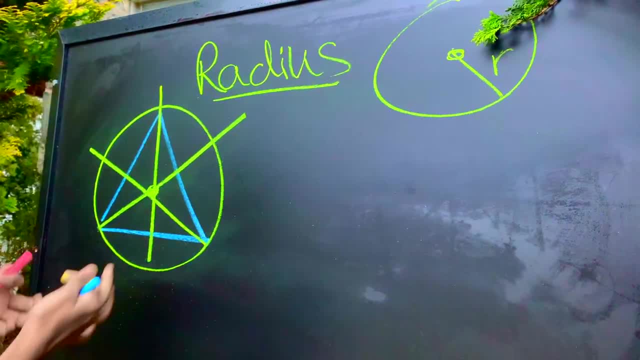 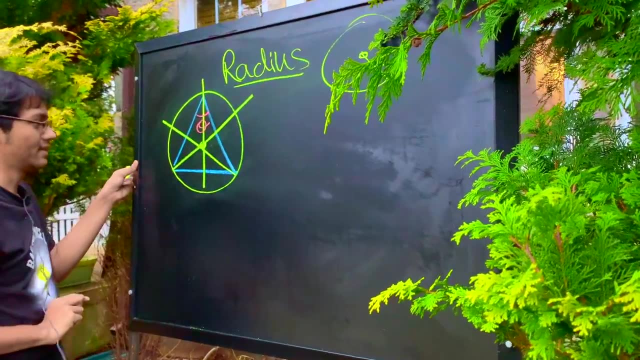 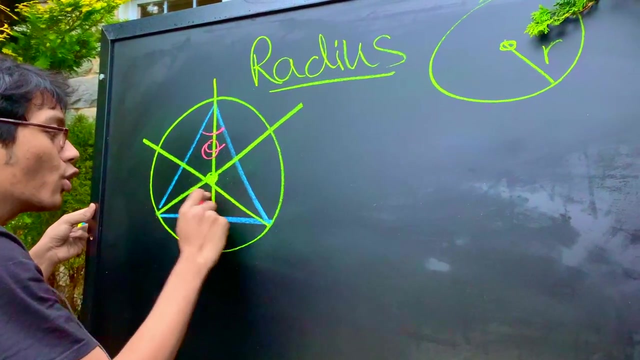 that radius. let's start by defining some angles. Is there any angles we can define here? Well, yeah, Look up here, There's an inscribed angle in the circle. Let's call that angle theta. Well, if this angle is theta, we know the central angle has to be two times that angle. So this whole angle here. 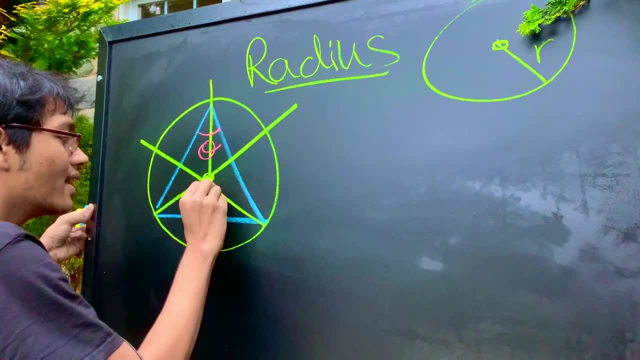 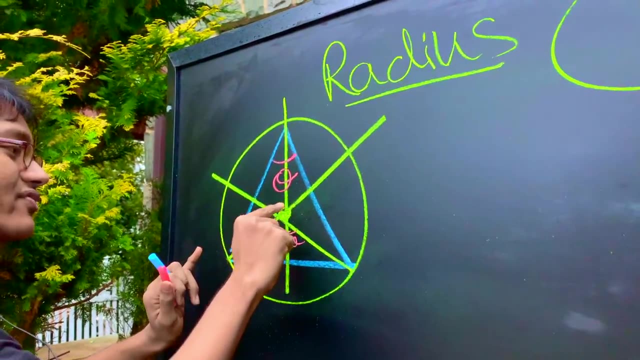 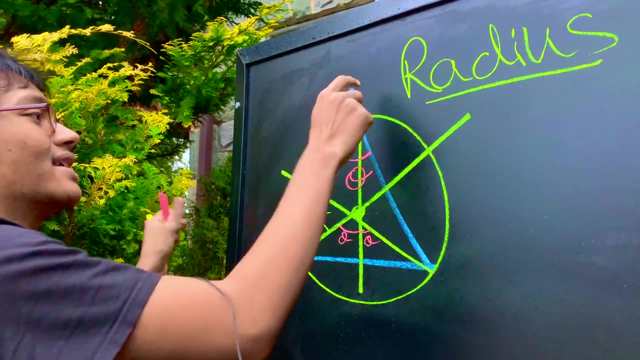 is two theta, But if we cut it in half it becomes theta and theta. Okay, so far, so good. you say. Now what can we do? Well, we know the distance from the center to the circumcircle- The circumference is going to be the radius r- and we know we can define this vertex as a. 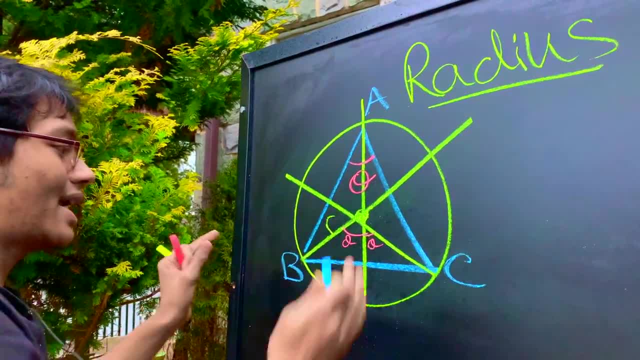 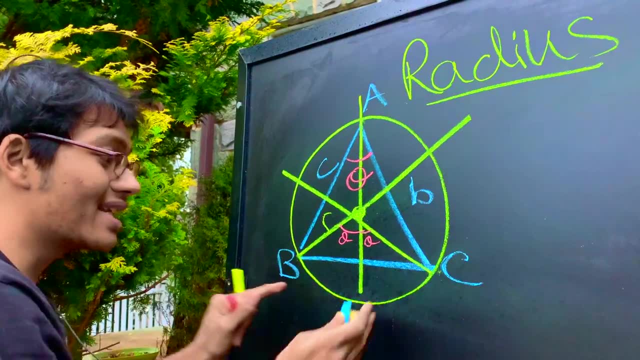 this one as b, this one as c, so that the length of this side we can say small b, the length of this side we can say small c and the length of this side is small a. But if we cut up this side, 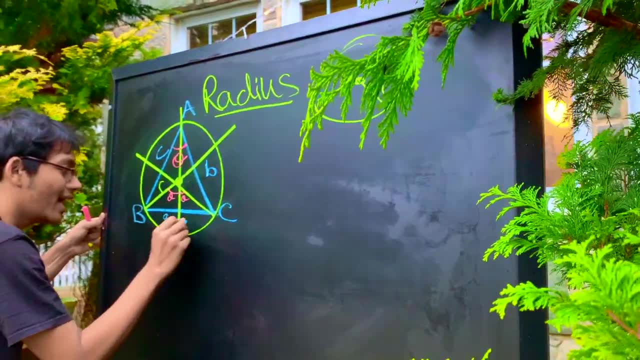 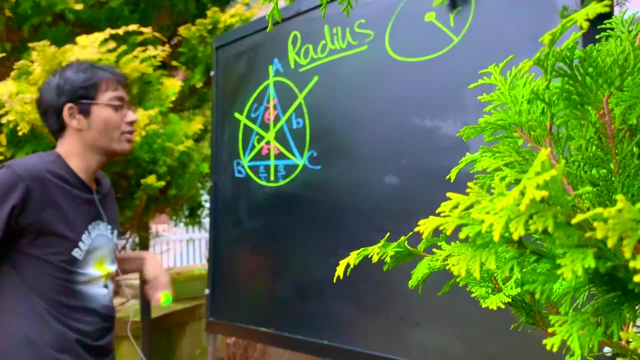 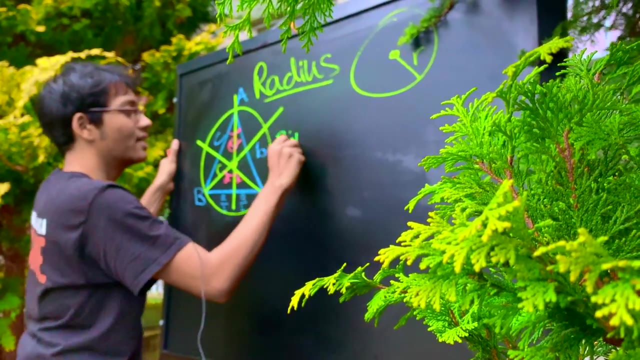 in half. well, what is small a divided by half? Well, it's going to be a over two, Okay. well, now we can use some trigonometry to our advantage. What trigonometry can we use to find the radius? Well, check it out. We can use sine of theta. What is sine of theta? 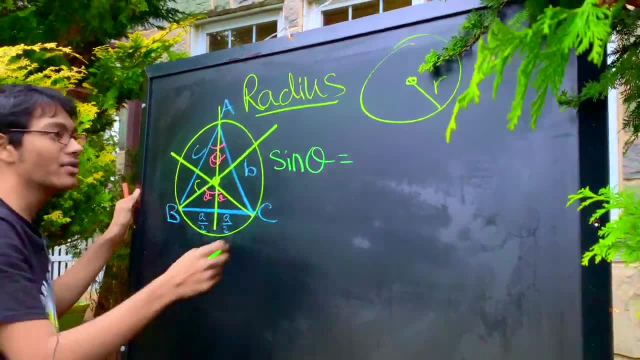 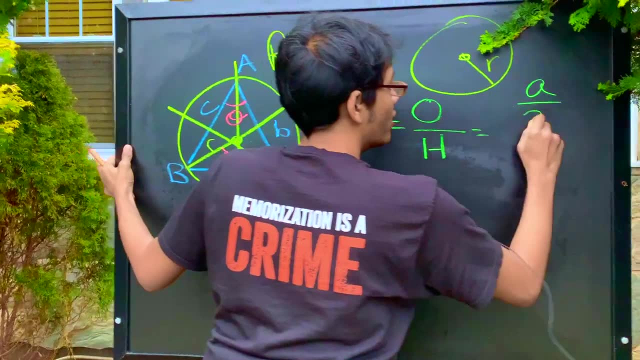 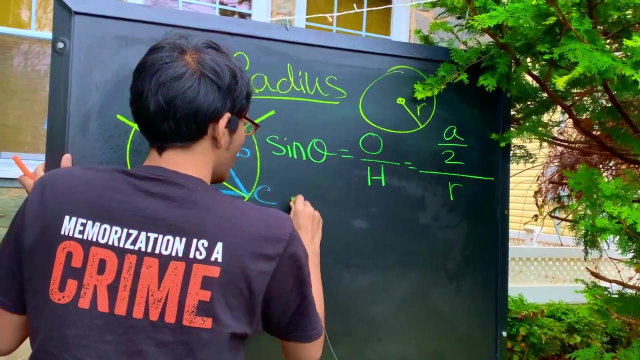 Well, sine of theta is opposite over hypotenuse. What's our opposite? It's a over two, A over two. What's our hypotenuse? It's r. And so if we isolate r, what do we get? r is equal to a. 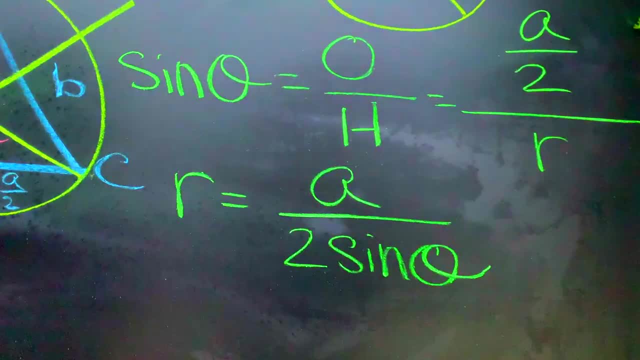 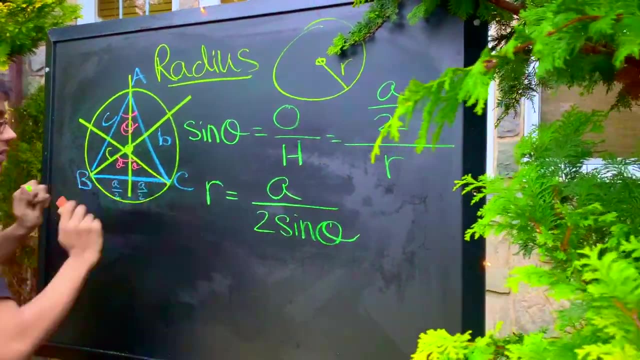 over two sine of theta, theta. Okay, so far, so good, you say, But we're not done. We can make this even nicer. Check it out: If we draw an altitude from angle c to the opposite side, here's that altitude, And what does. 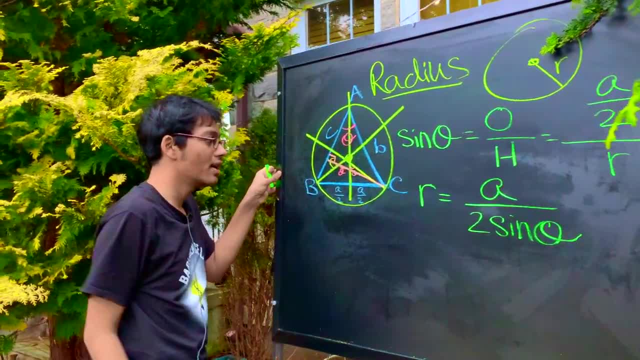 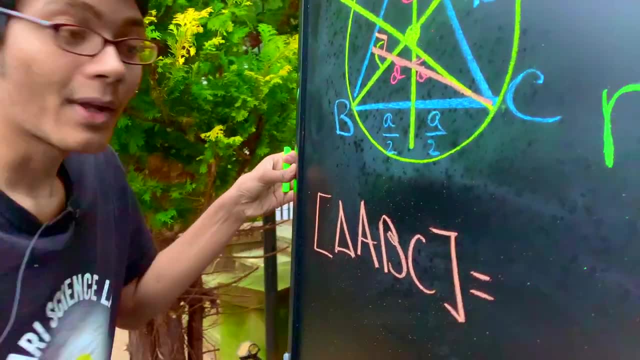 that altitude do. Well, it gives us a right angle, And so we can use that to our advantage, because now we can say: the area of our triangle, abc, is what Our areas have, bh, as I'm sure you know by now. And well, what's b? What's our base? 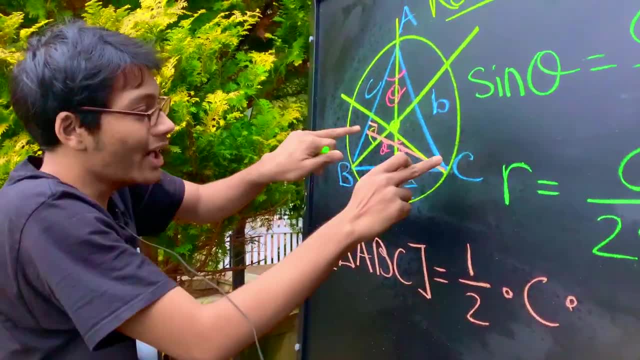 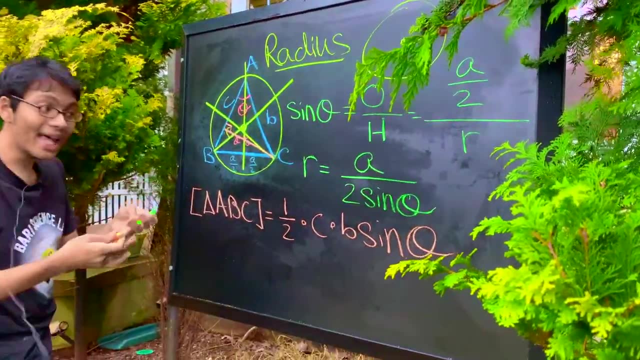 Our base is c. You see that It's c. And what's our height? Well, our height is going to be this. But what's this? This is just b sine of theta. b sine of theta. Well now, if you look carefully, 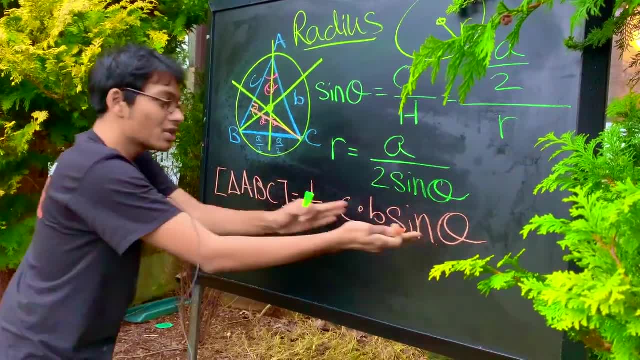 we're almost done. We're almost there. How are we almost there? Well, we can solve for sine theta here and then plug in. So what's sine of theta? What's sine of theta? Sine of theta is equal to. 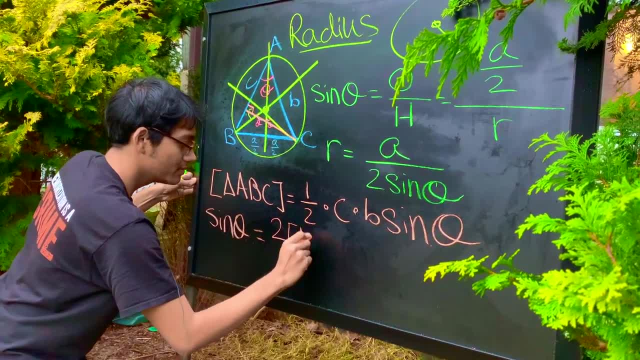 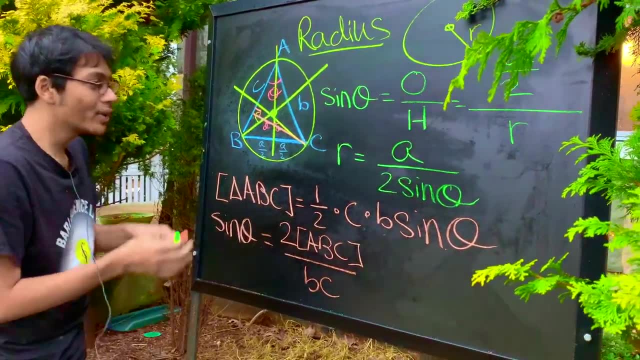 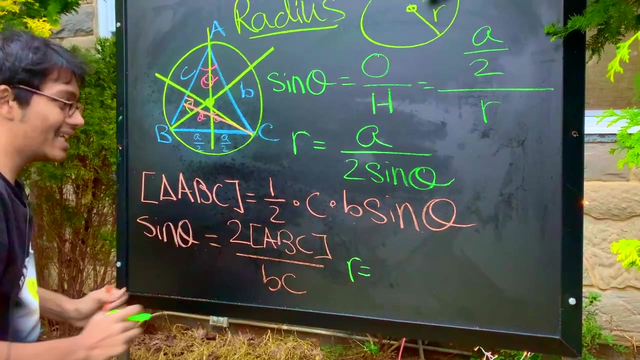 what It's two times the area of the triangle divided by bc. bc. And now, finally, we can conclude what the radius of the circumcircle is going to be, The radius of our circumcircle. if we take this sine theta, plug it back in, what are we going to get? 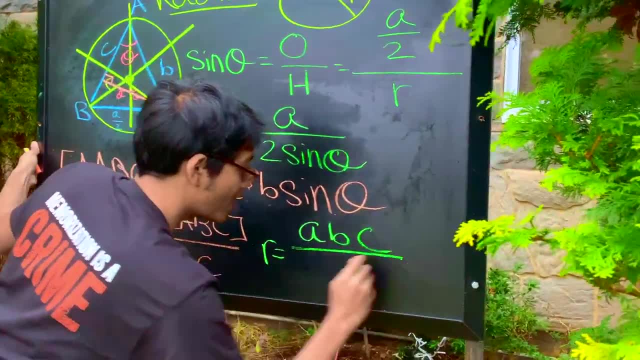 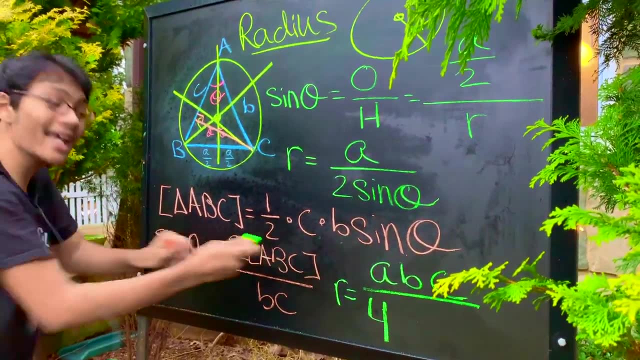 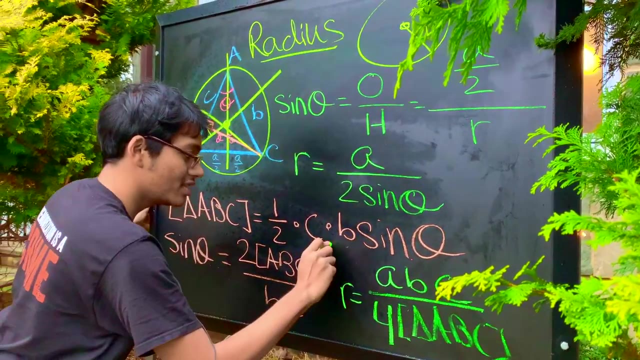 Well, we're going to get the product of all three lengths of the triangle divided by what Well? two times two, that's going to give us four, Four. what Well? four times the area of the triangle, Four times the area of our triangle, Triangle a, b, c. And that, ladies and 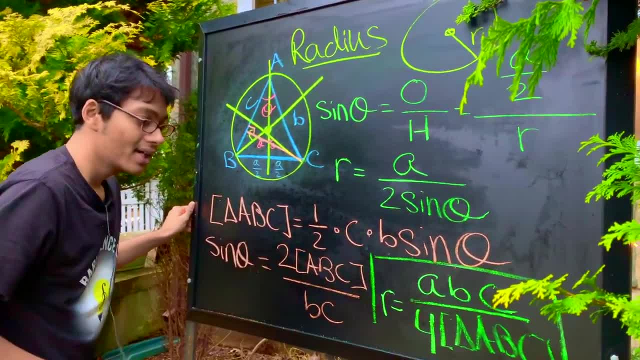 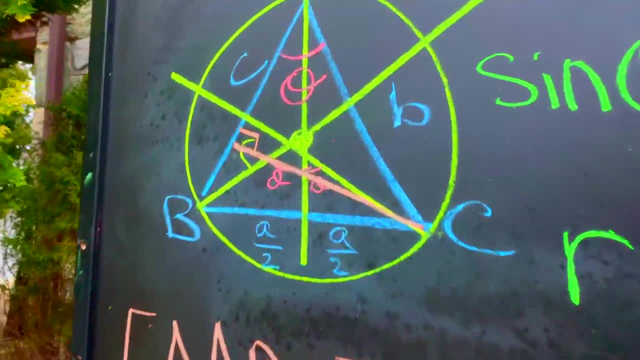 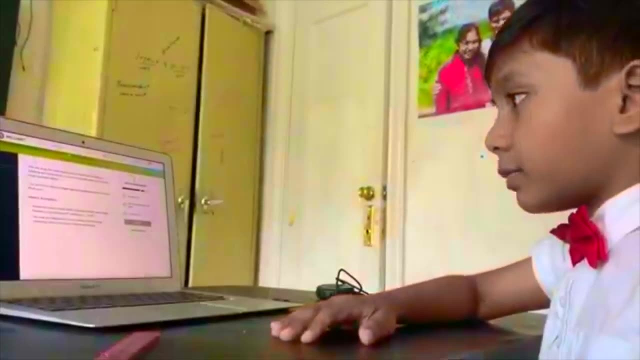 gentlemen, is the formula we've been looking for The area of the triangle given in terms of the circum radius. Thanks for watching this lecture of Math, for One sponsored by Brilliantorg, and we'll see you next time. Ambition plus MKO plus scaffolding equals learning. We believe anyone can learn anything. 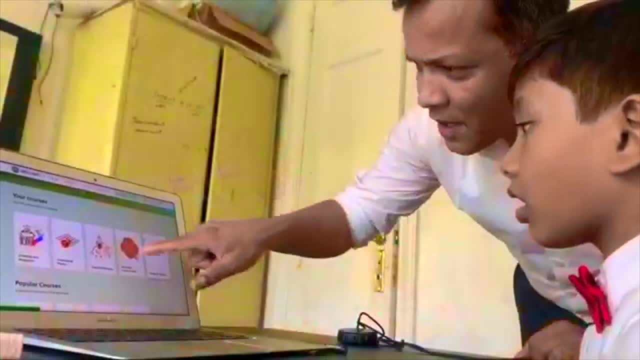 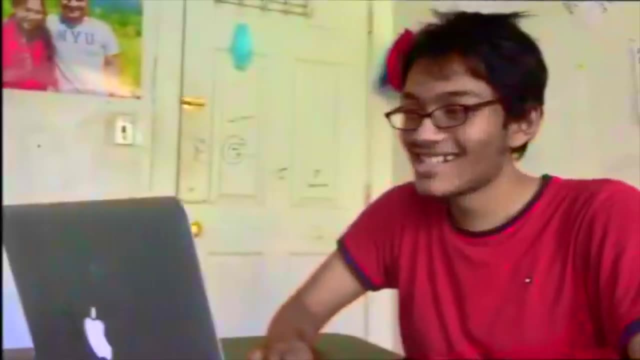 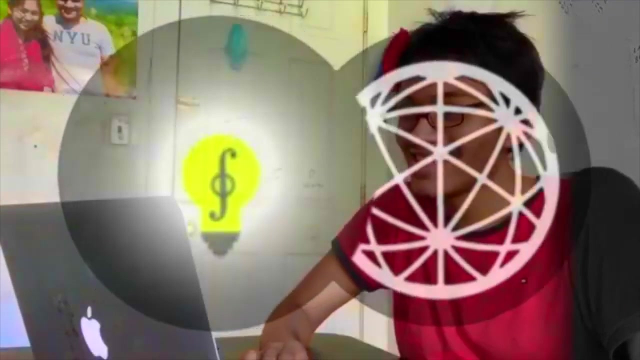 That's why our motto is: memorization is a crime, And that's why we partnered with Brilliant. Brilliant transforms math and science into hands-on activities so that you, too, can understand everything from first grade. math to E equals MC squared, Barry Science Lab, and Brilliant is your.